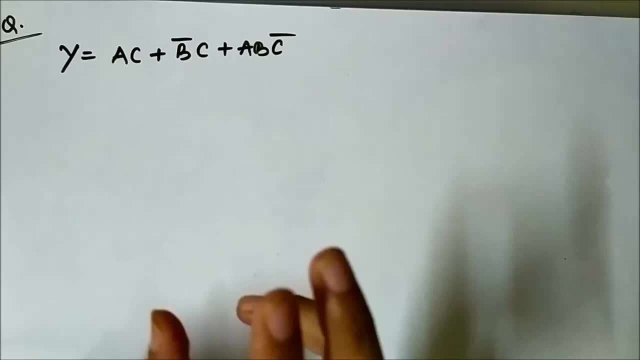 increased the number of terms and there are three signal values. So far the questions which we have discussed, it was a simple expression involving two, three or four signal values. but it was a simple expression involving two terms or one term. But here we have three. 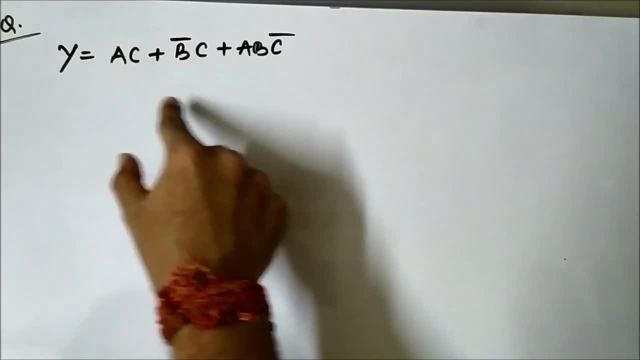 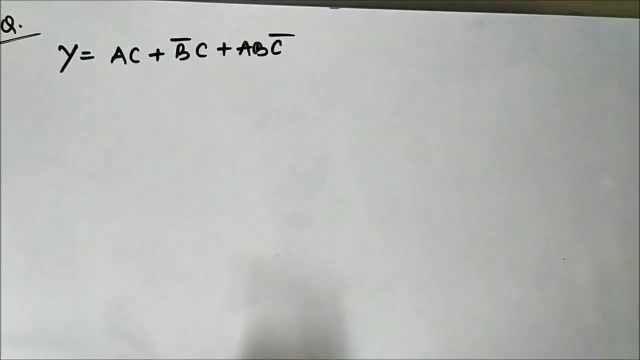 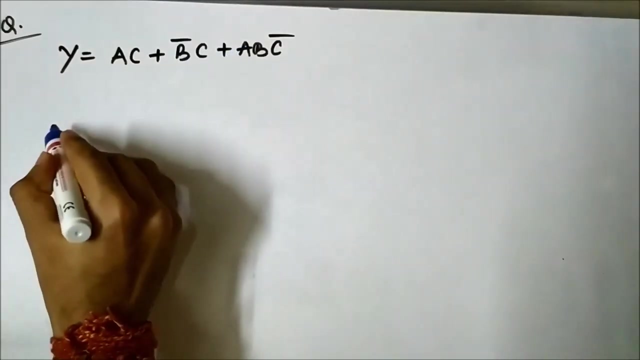 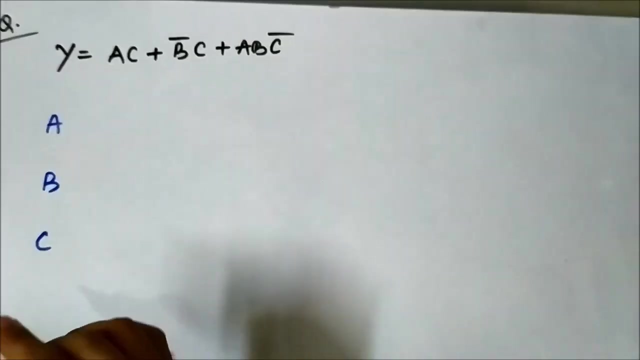 signal values a, b and c. but there are three terms as well: a, c, b bar, c, a, b, c bar. So this is a new thing. So let us design it. So: first we will assign the different signal values a, b, c, then by: 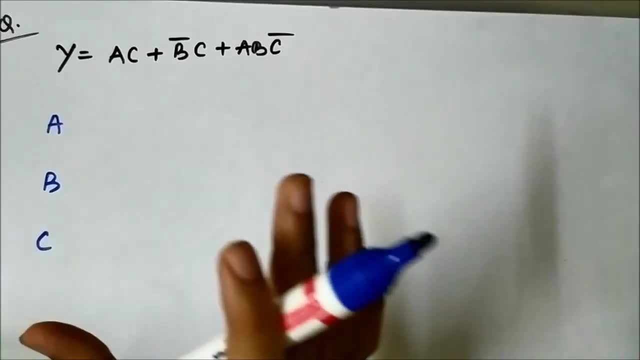 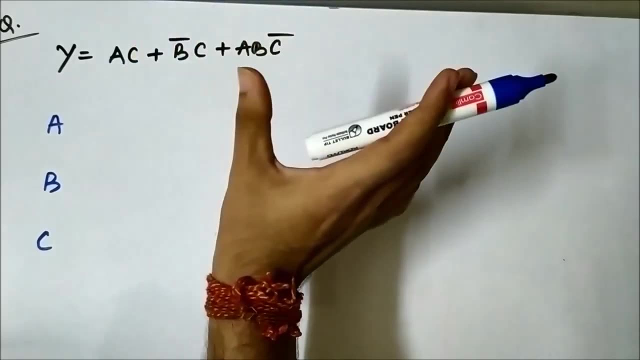 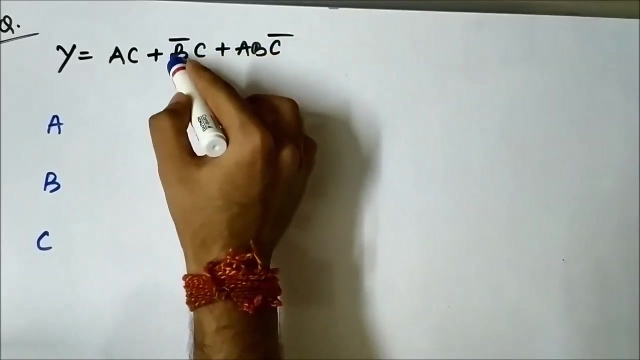 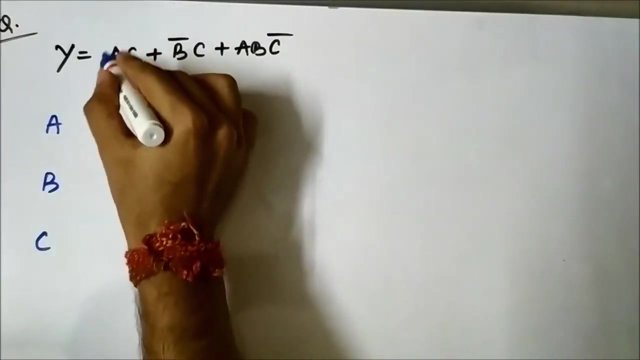 looking at the expression we will try to figure out which logic gates will be required. So here there is a AND operation between a and c. So AND gates will be required. The plus sign indicates OR gates will be required. So first we will target each term separately. We will try to get each term separately and 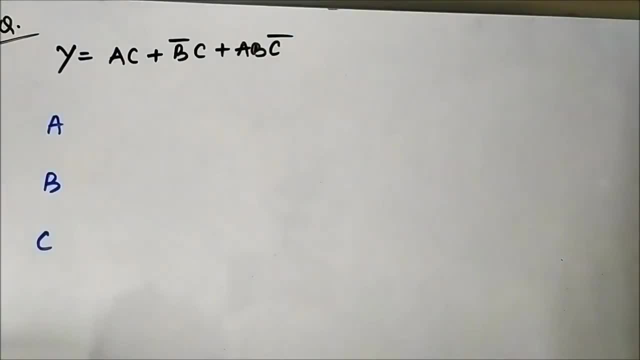 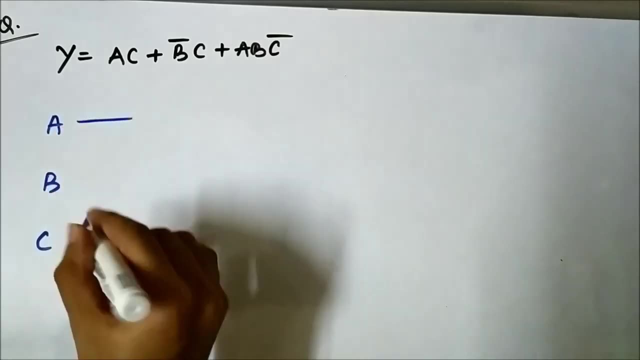 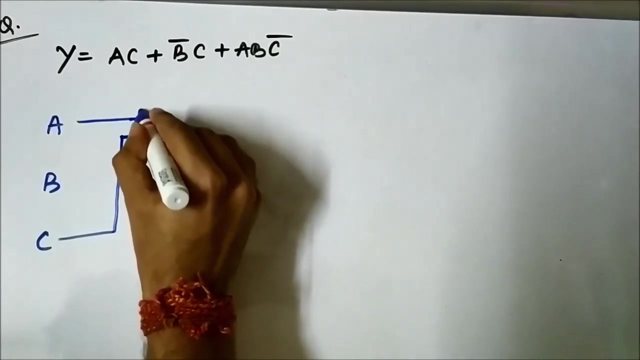 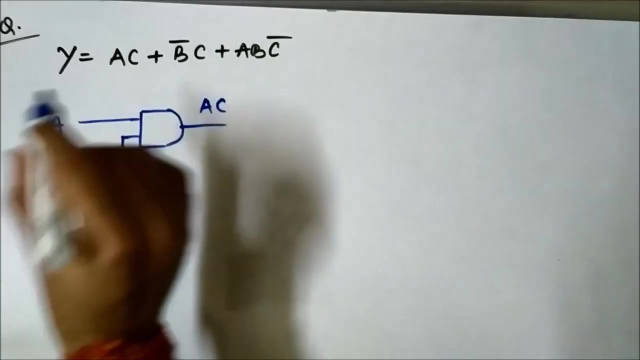 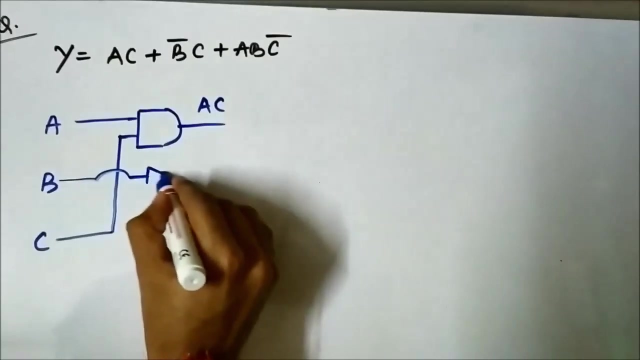 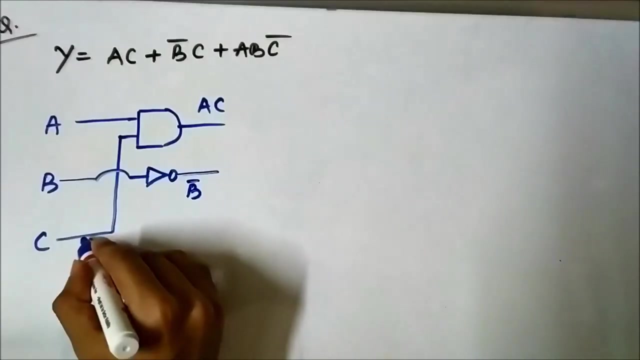 then we will combine them together, First a and c AND operation. So we will give a and c AND operation to a 2 input AND gate to get ac. Then is b bar c, So for that b is passed through an inverter or not gate to get b bar. Then it is ANDed with c, So 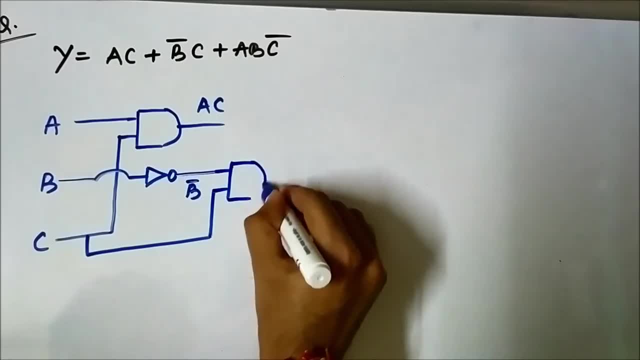 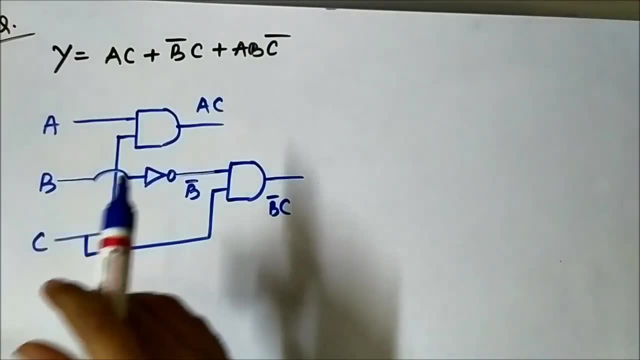 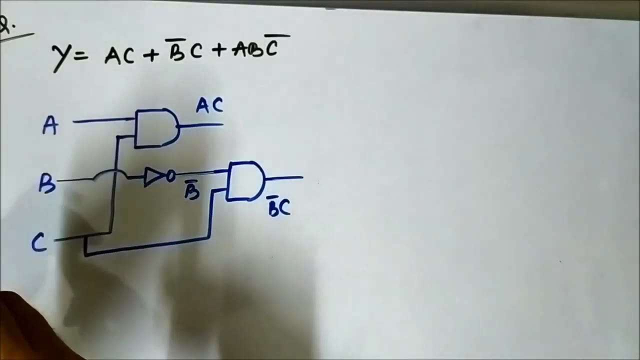 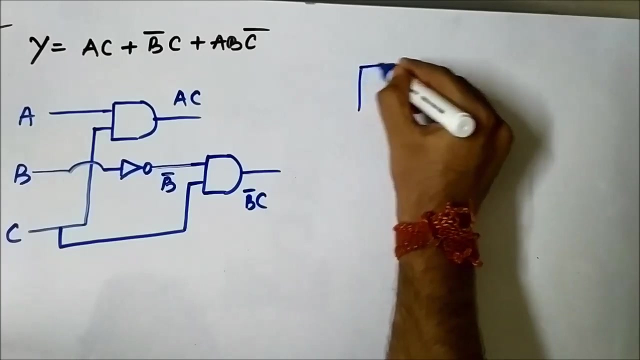 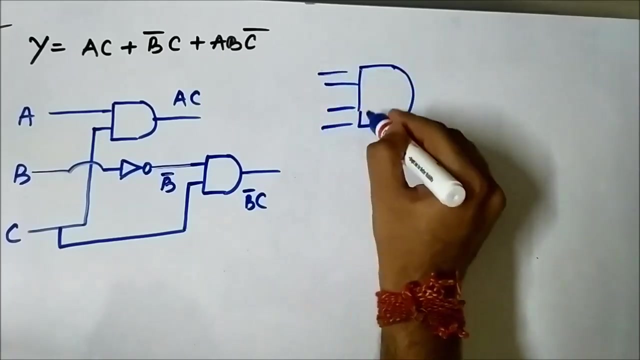 to get b bar c Now this a b, c bar. Now here the question is: it depends on what is being given in the question. Now we have logic gates which can have three inputs. Multiple input logic gates are available. It can have two inputs, three inputs, four inputs, five inputs. 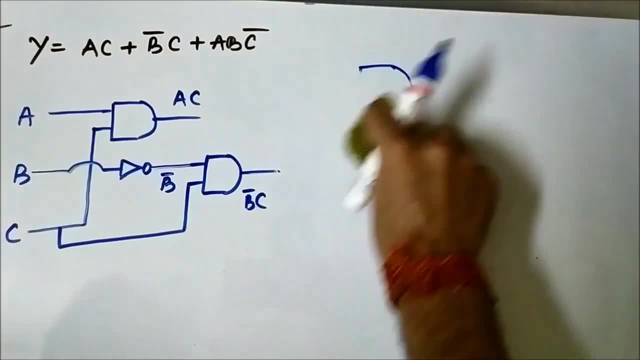 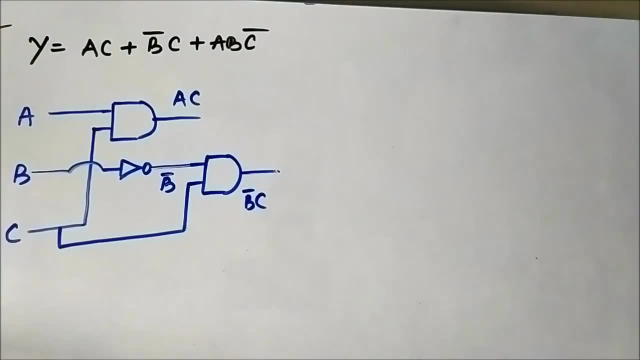 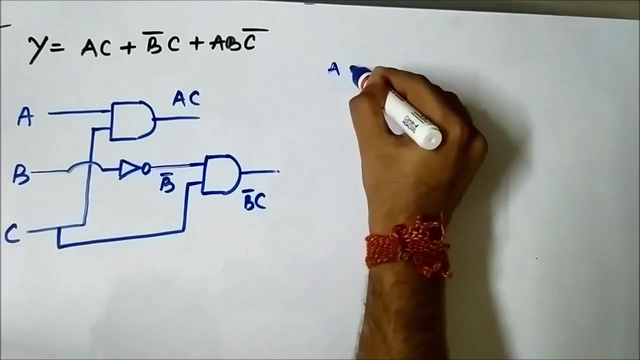 whatever. So if in the question it is being given that you can use a three input and gate, or a three input or gate, or a three input, whichever gate, then you can directly do this by just that: a, you give a, you give b and you give c with an inverter. 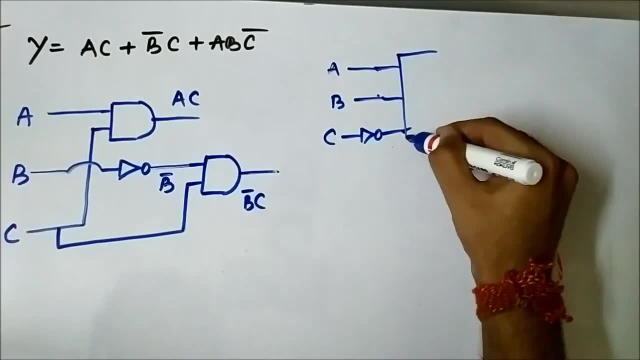 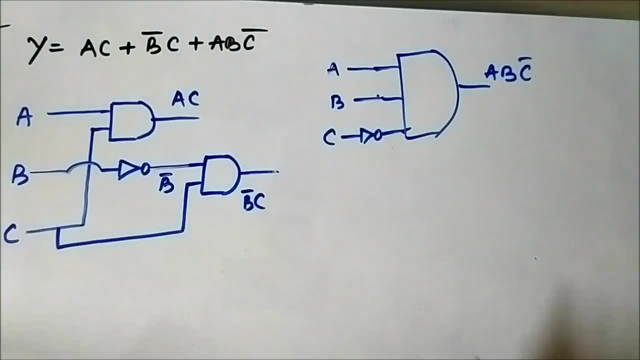 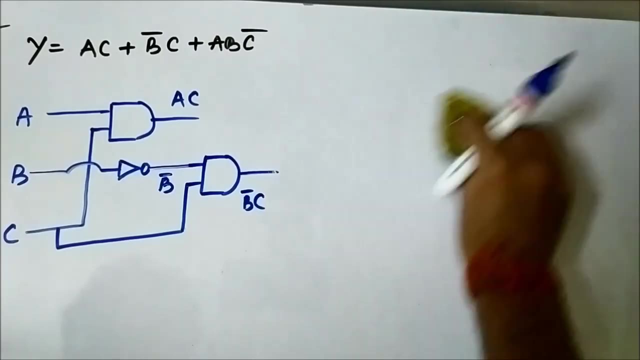 To a, three input and gate and we will directly get the expression a, b, c, bar. But here nothing is been mentioned like that. So we cannot use a, three, input and gate, So we have to do it in steps. So how we will do it, Let us see. So first we will have to get a b, First we will 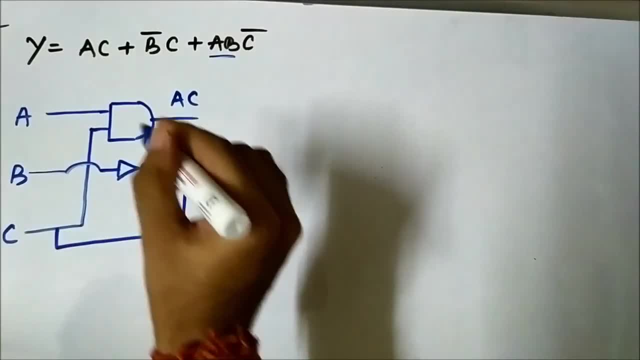 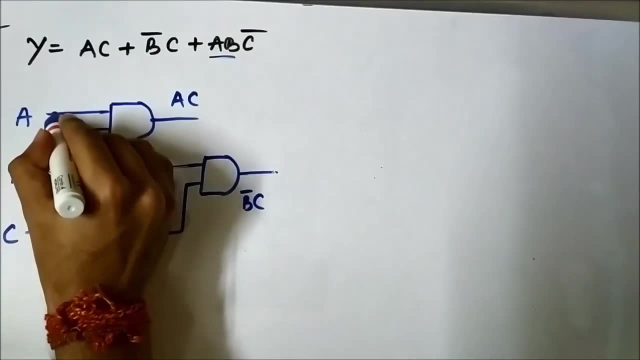 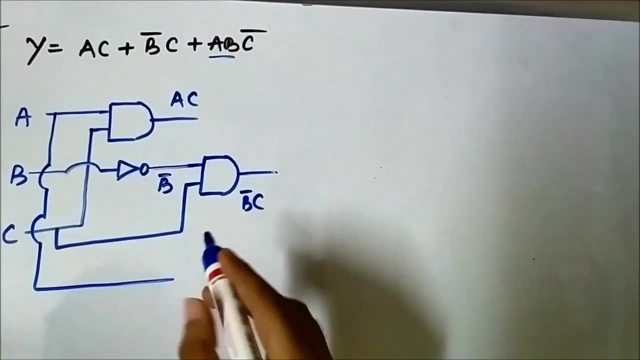 have to get a, b. So for that you take a here. So it can get a little bit complicated, So confusing here. So you follow me carefully. We will take a first. So this is a, We will give it. 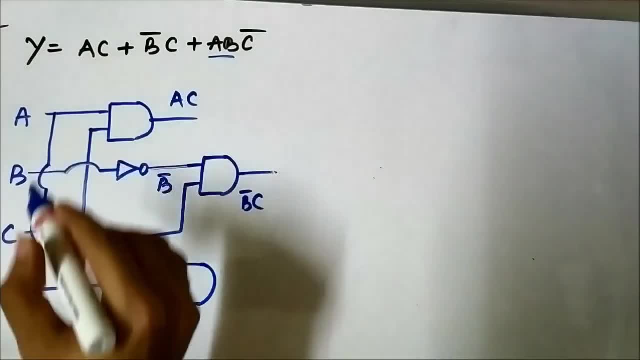 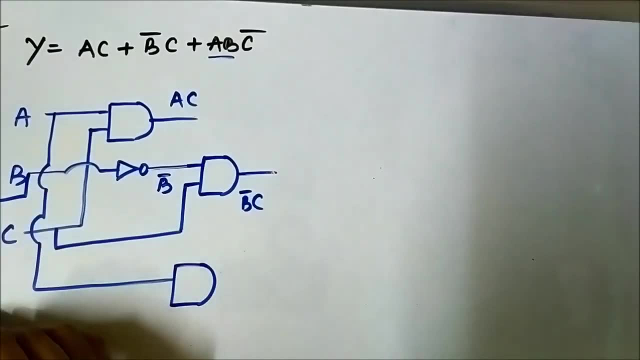 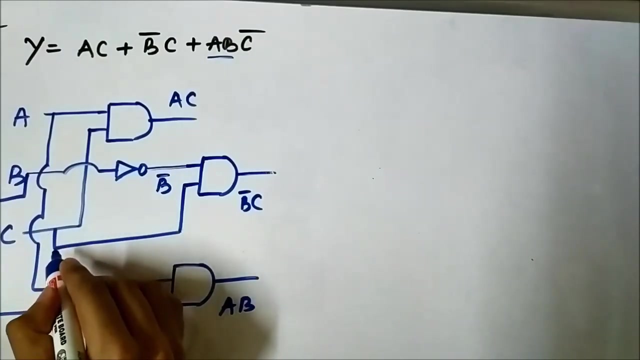 to a, two input and gate a, and then we will get b. So I am taking b from here, a and b. So this gave us that b. Then c for c bar. we will have to take c here from here. we will pass it through. 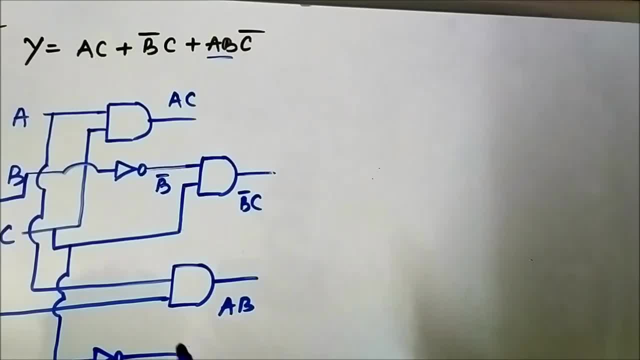 an inverter, we got c bar. Now we have 2, and these 2 a, b and c bar give it to a 2 input and gate to get a, b and c bar, All right. So the thing is the. 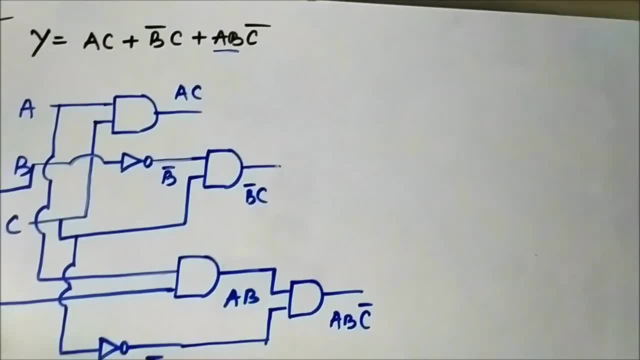 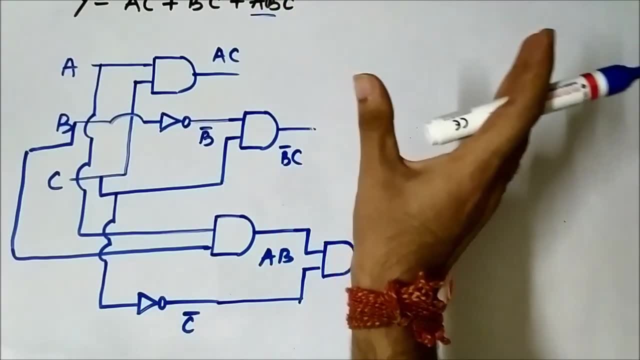 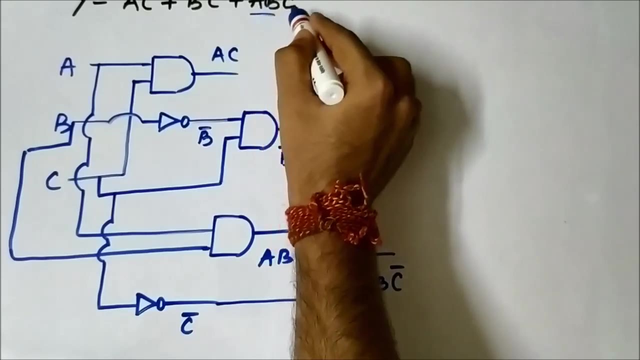 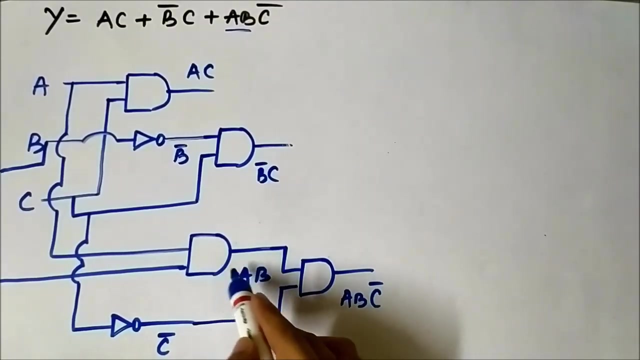 a, b, c bar. okay c to get a b, c bar. we cannot use a three input and gate here, because nothing has been mentioned like that. we can only use two input gates. so for that we have to break it into two parts. first we'll have to get a- b. so we took a b, gave it to a two input and gate. we got a b. 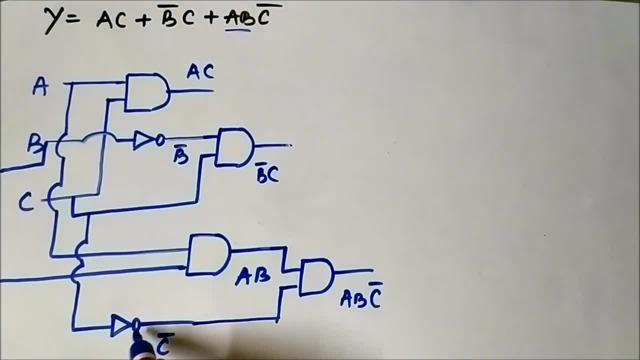 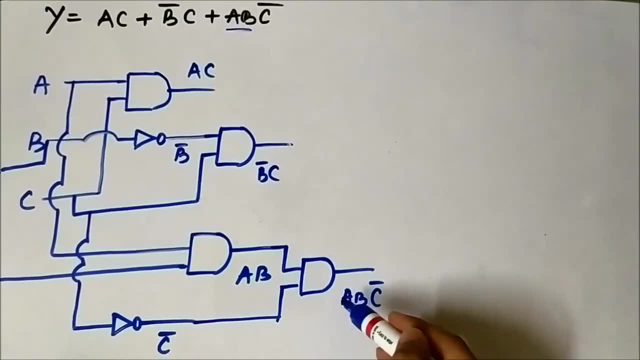 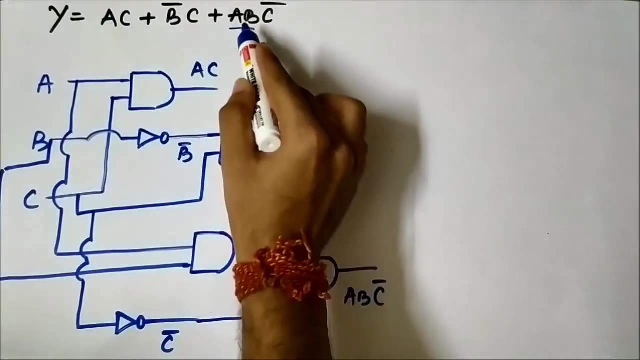 then we took c signal, passed it through an inverter or a, not gate, to get c bar. then we added a b and c bar to get a b c bar. okay, in this way we got a b c bar. now we have got all the terms. we have got a c, we have got b bar c. we have got a b c bar. again. the question here: if we are permitted, 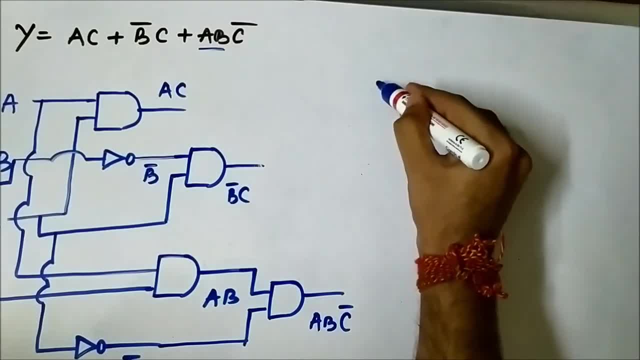 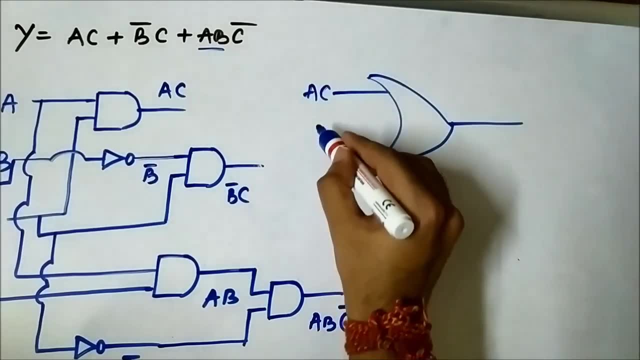 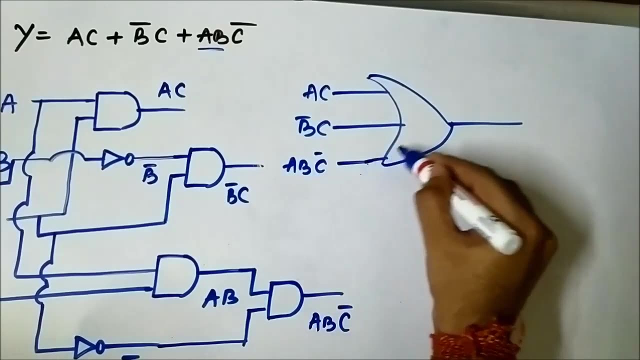 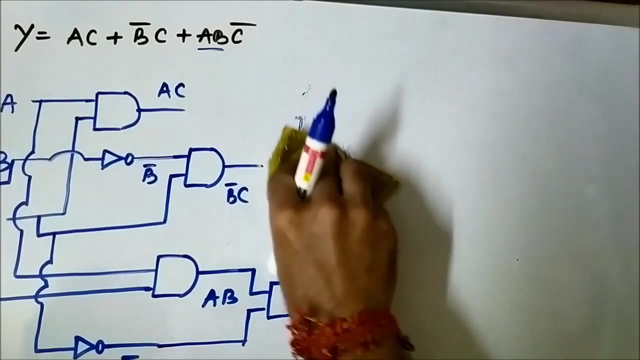 to use three input gates, then we can directly pass it through a three input or gate a c then b bar, c then a b c bar. we can directly pass it through a three input gate and we will get the output directly. but here we are not. there is nothing like that mentioned in the question, so 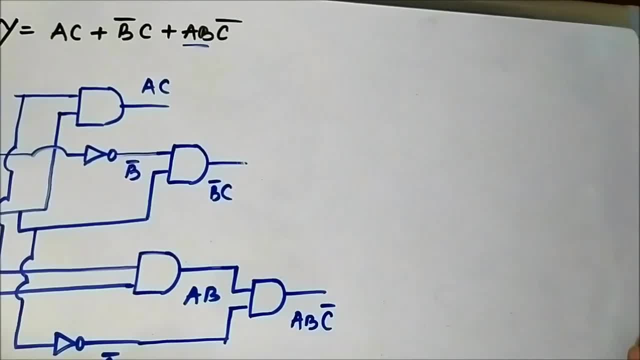 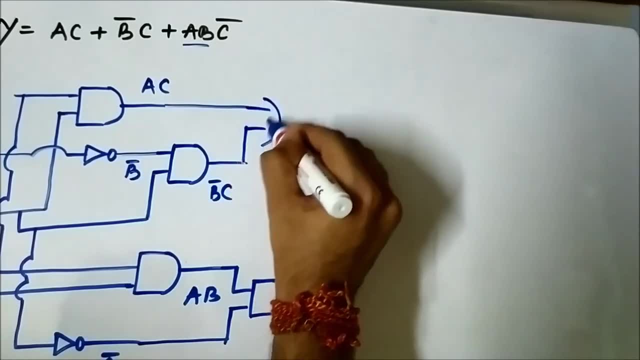 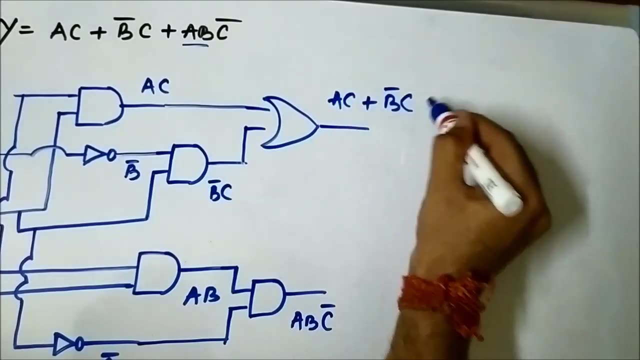 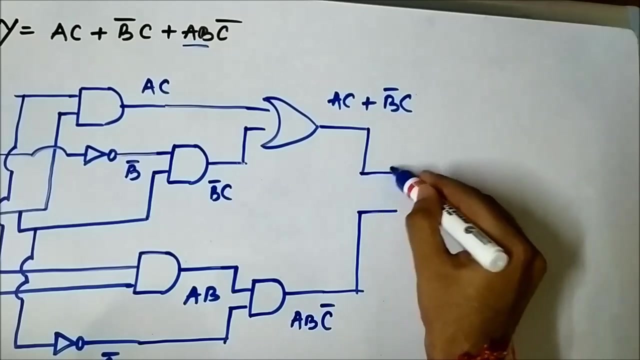 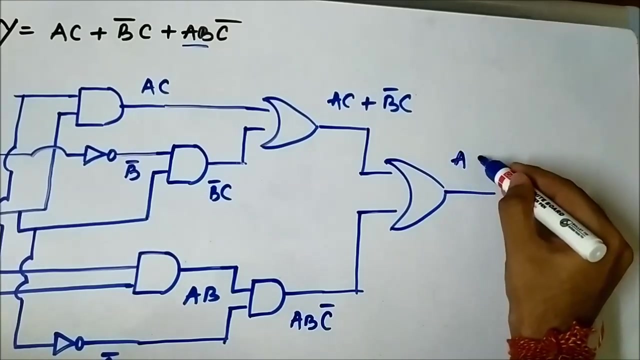 we have to go by the two input gates. okay, so for that, first we have to pass these two terms through: a two input or gate, which will get a c plus b bar c. then we'll pass this output with a two input or gate, which will get a c plus b bar c. 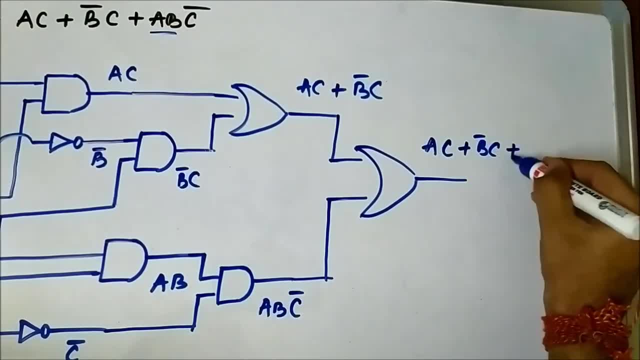 plus a, b c. bar plus here means or operation. okay, so we have to go by the two input gates and we will get a c plus b bar c. then we will pass this output with a two input or gate. okay, so we have to go by the two input gates and we will get a c plus b bar c. then we will pass this output with a two input or gate. 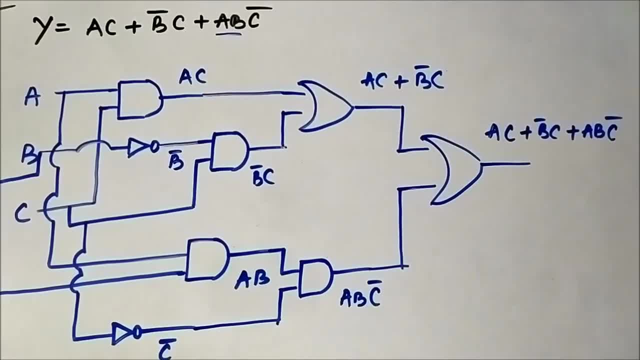 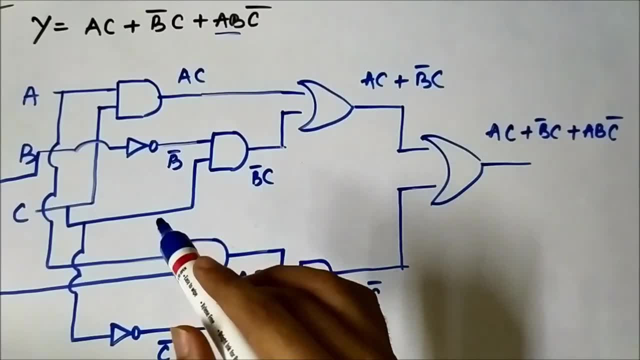 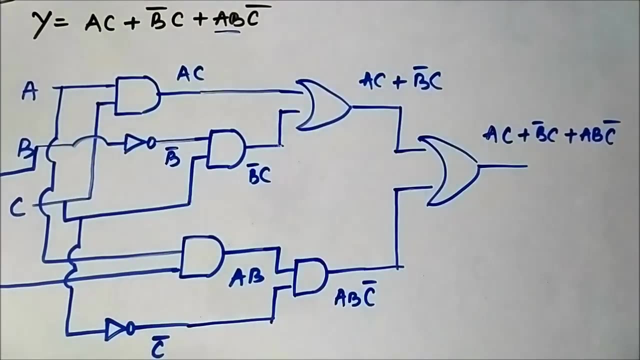 so this can be a little bit confusing for you. so you follow the steps carefully, you pause the video at any instant where you do not understand, again rewind it and watch it, because a lot of connections have been made here. so i deliberately took this question because of a lot of concepts that are involved here. 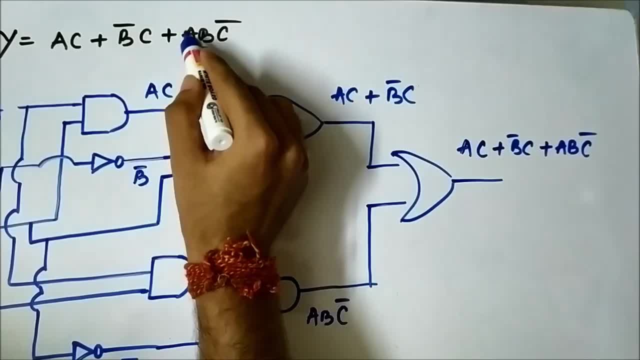 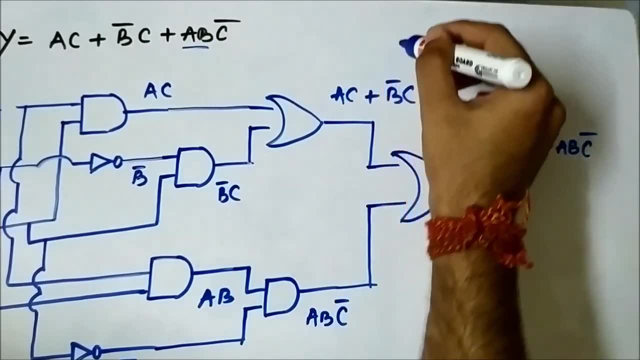 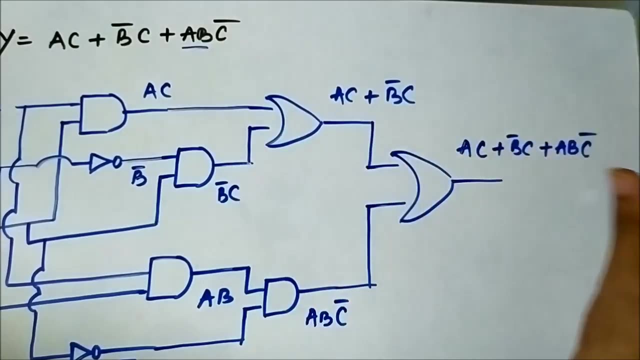 here it involves three signal values and three terms. here we have a three, a term involving three signal values, and i deliberately told you that we cannot use a three input gate directly because it has not been mentioned in the question, so we have to go by the two gate concept.